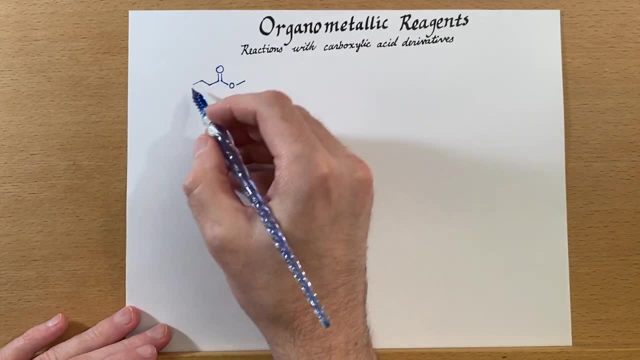 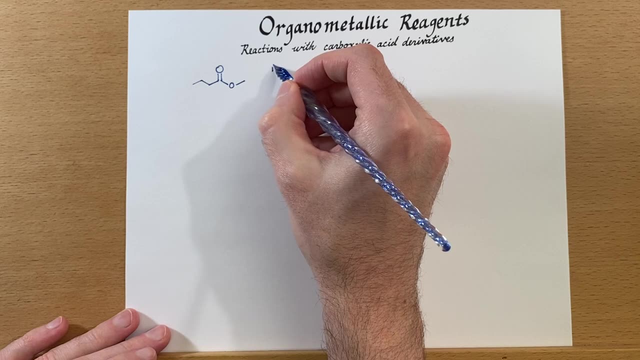 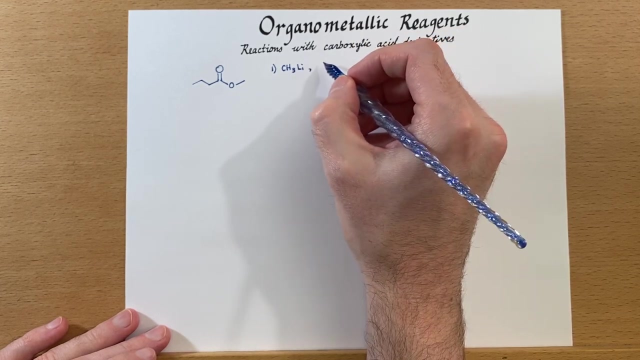 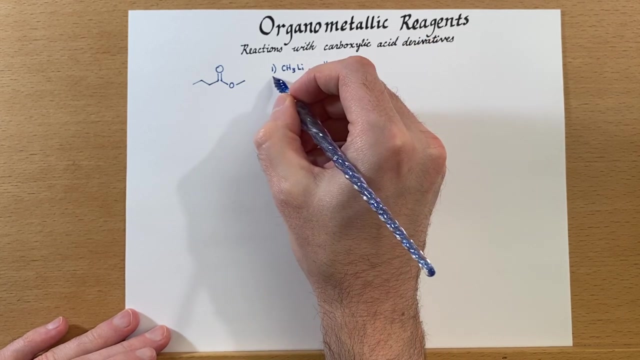 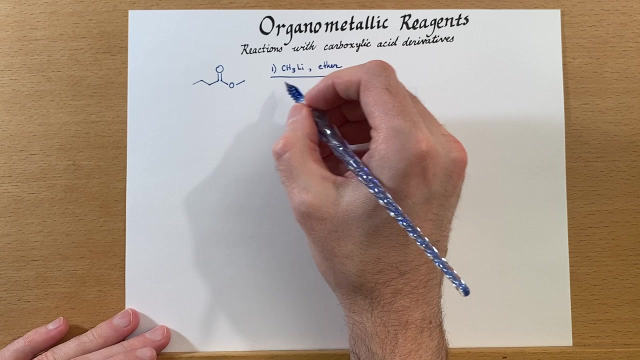 So here we have an ester And let's react it with methyl lithium, And of course we'll need an appropriate solvent for this And some kind of ether will work And you may wish to have a lower temperature, But this reaction is going to go quickly, otherwise 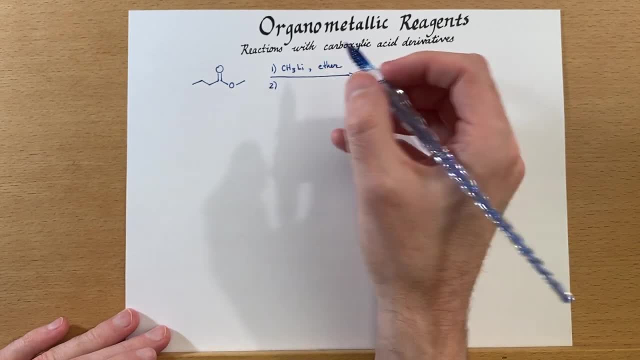 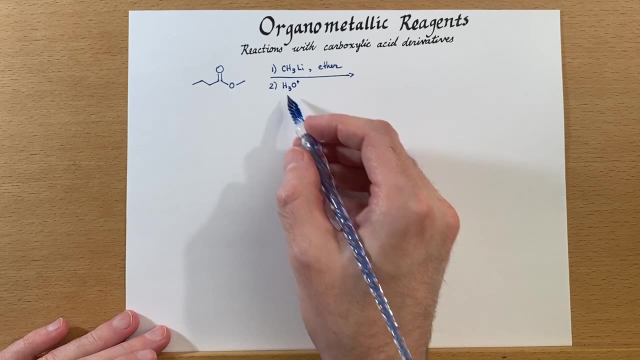 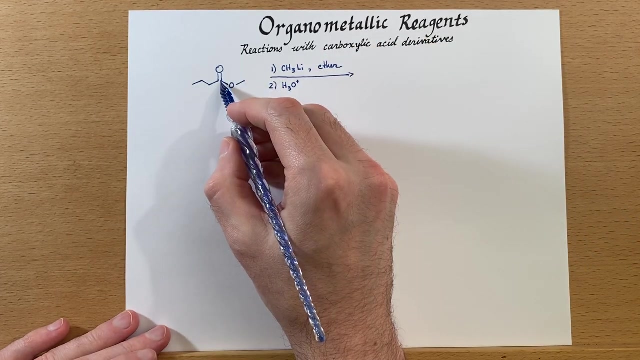 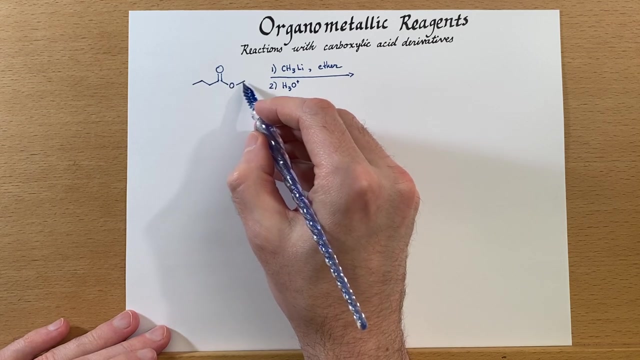 And then, after this reaction is over, we'll need an acid workup. So I'll just write H3O plus to indicate acid workup. Now, when we do this, this will add to the carbonyl And then our leaving group right here, the alkoxide methoxide group, is going to depart. 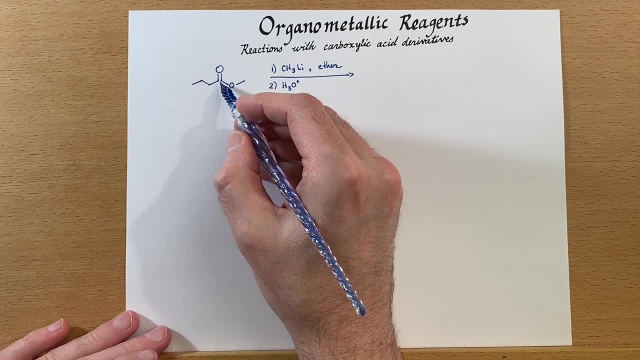 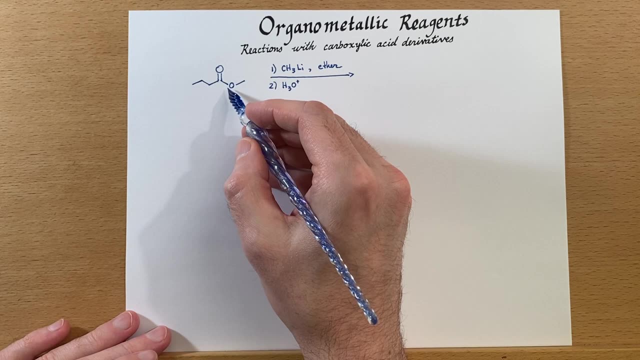 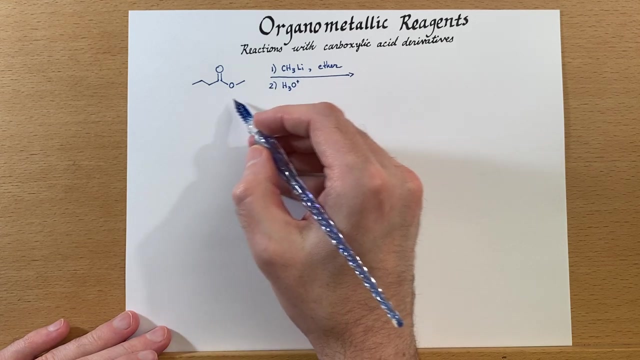 At that point we would be left with a methyl group on the ketone, So we would be left with 2-pentanone. Well, 2-pentanone will also react with the organolithium reagent And we'll get another addition. 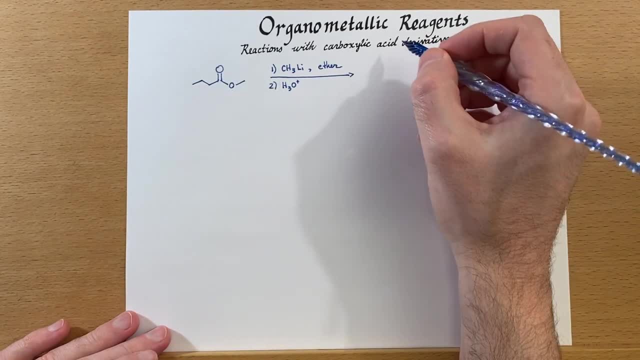 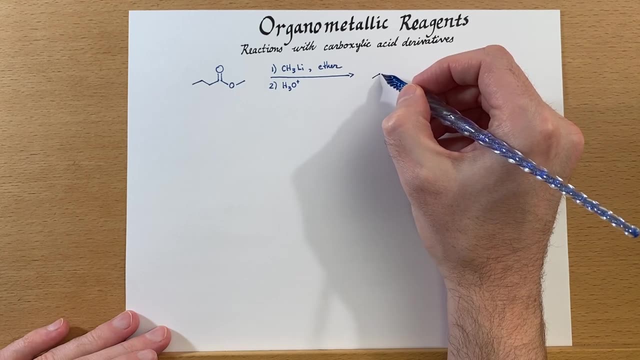 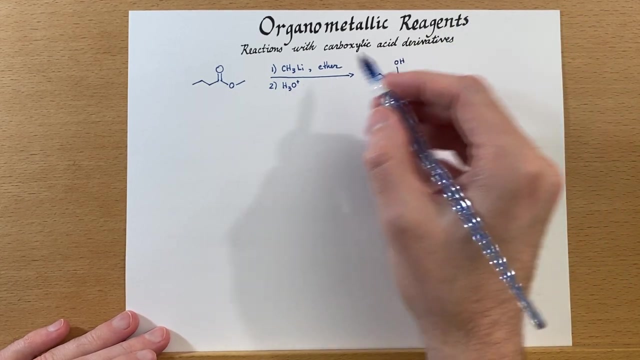 And then that will open up the ketone, And then we'll open it up and form an alcohol there. So what we'll see is there will be two equivalents of the organolithium reagent added. So the acid workup step will produce the proton right here on this alcohol. 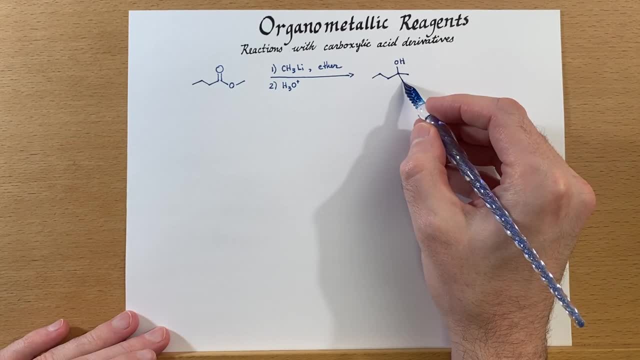 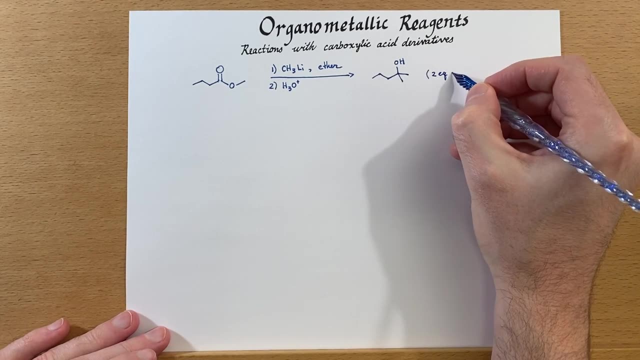 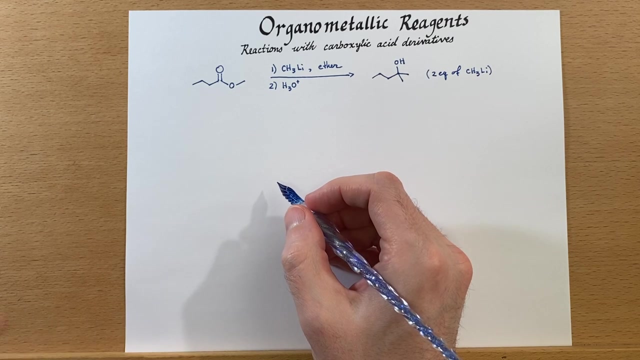 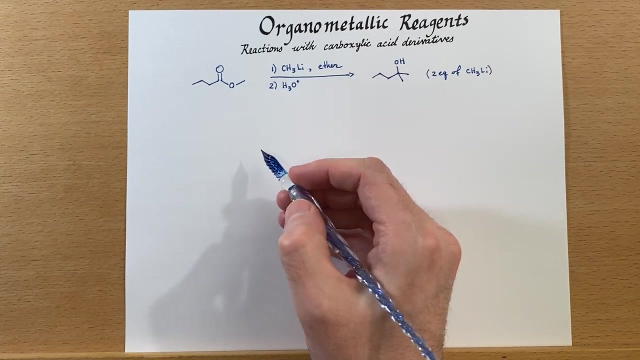 And we're going to have these two methyl groups added to that carbonyl. Now we'll see similar reactivity from acid chlorides and grignards, or esters and grignards for that matter, But my example is including an acid chloride. 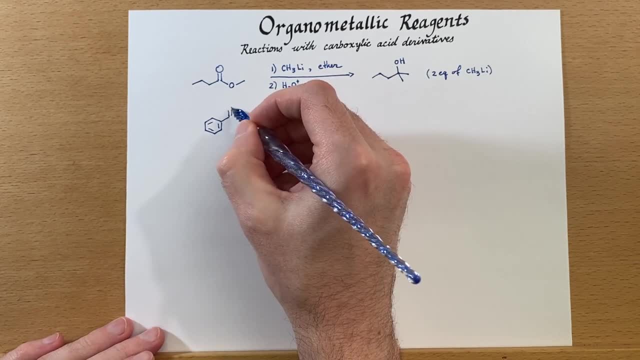 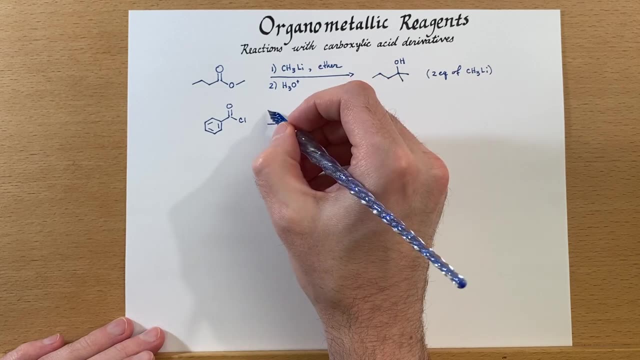 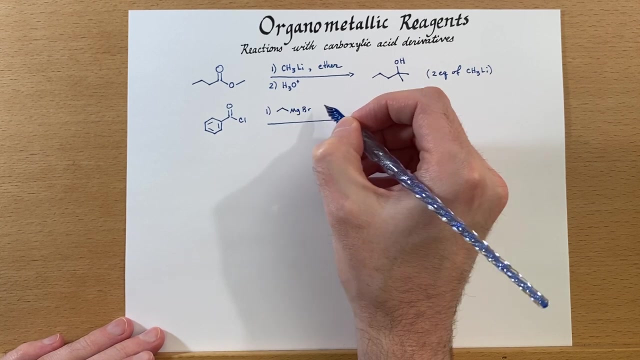 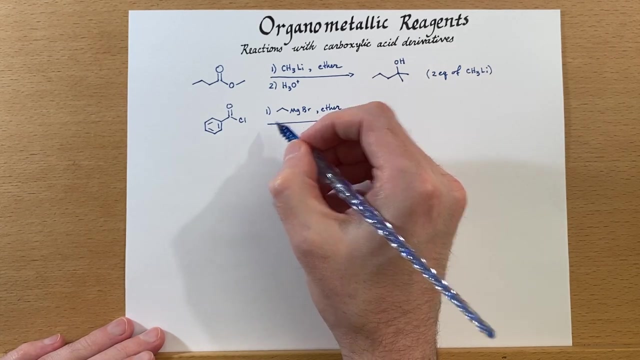 So we'll have benzoyl chloride, And if we add some grignard to it, let's go with the ethyl magnesium bromide, And of course we would need an ether solvent, And then again we'll need an acid workup. 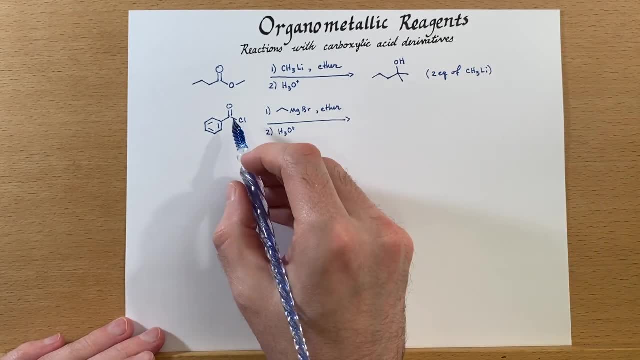 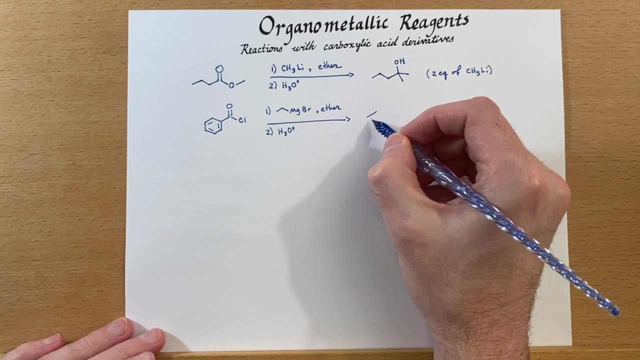 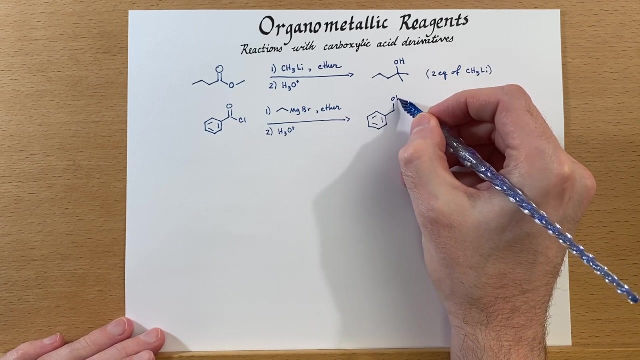 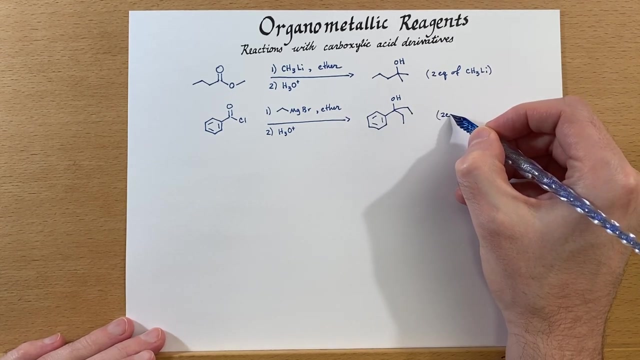 For this reaction we will also need an acid workup And we'll also be adding two equivalents of the grignard or the organometallic reagent to the compound And again forming a tertiary alcohol. So two equivalents of 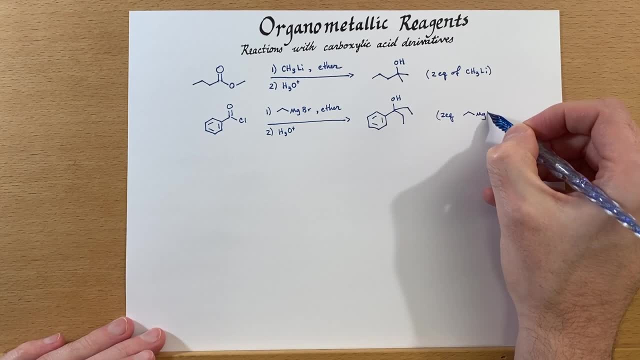 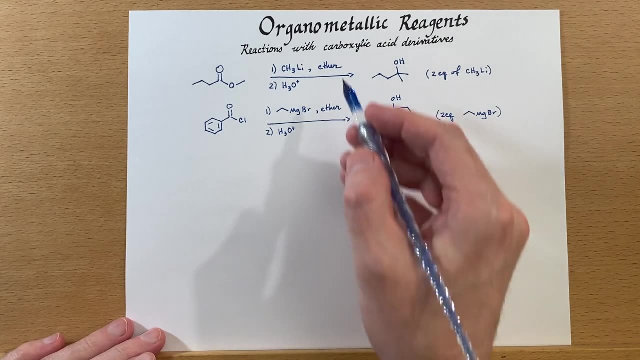 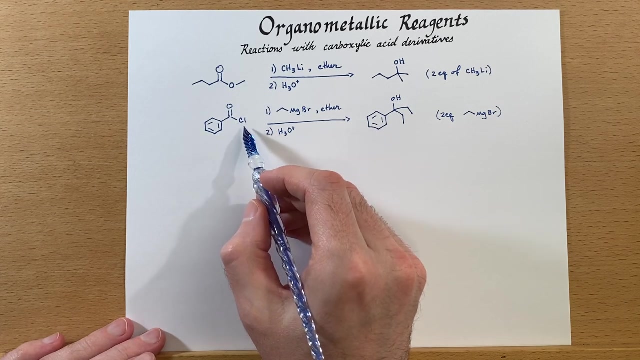 of the grignard added. Now, the mechanism for these are essentially identical. The only thing that's changing is the leaving group. So in this case, we have a chloride that's leaving. In this case, we have a methoxide group that's leaving. 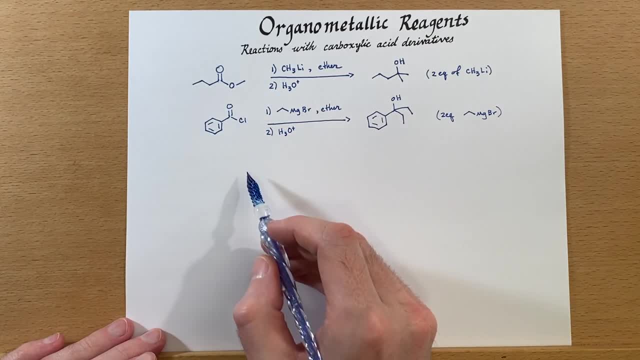 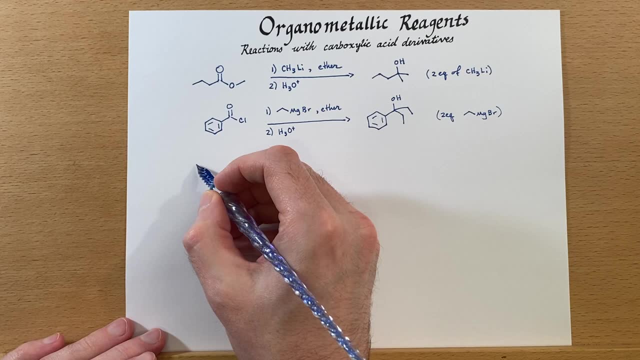 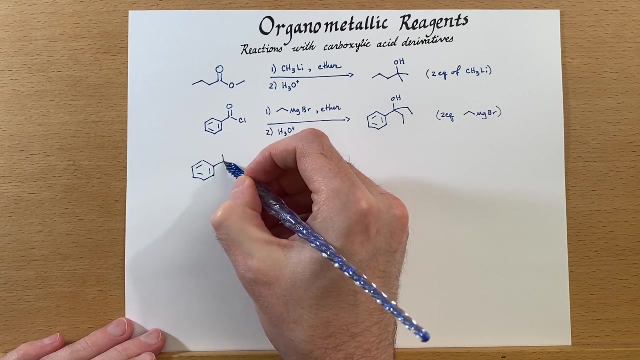 So we'll go ahead and go over the mechanism for this process And once we'll get halfway, you'll probably recognize the mechanism from previous videos where we had a grignard attacking a ketone. So we start off with our acid chloride. 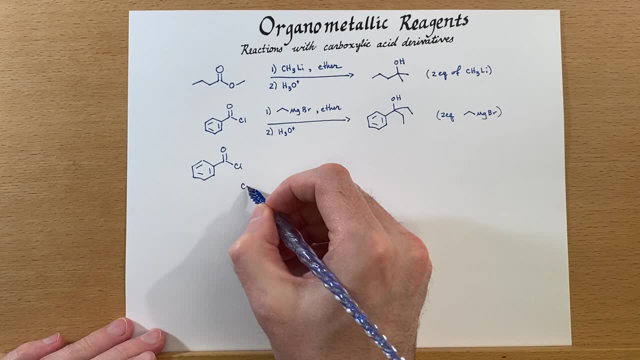 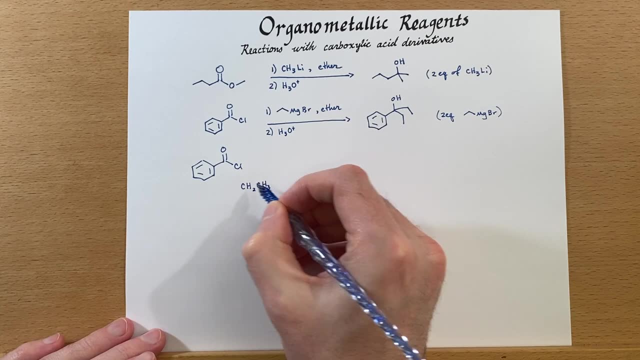 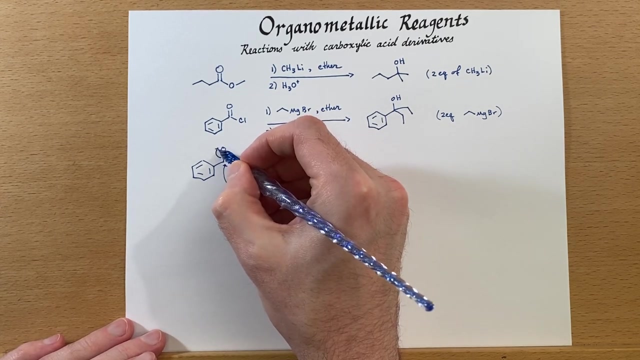 and our grignard reagent will attack the ketone Or the carbonyl, I should say. So there's our initial attack. Electrons move up onto the oxygen And next we have this intermediate reaction And next we have this intermediate reaction. 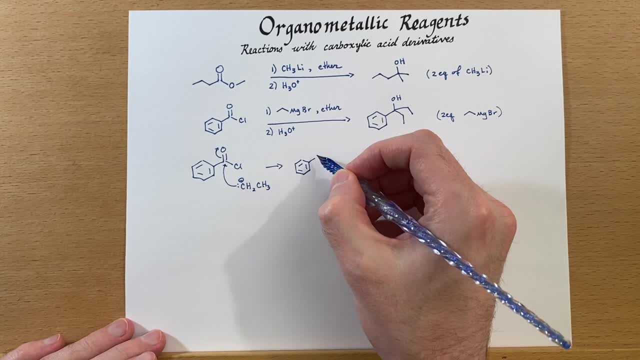 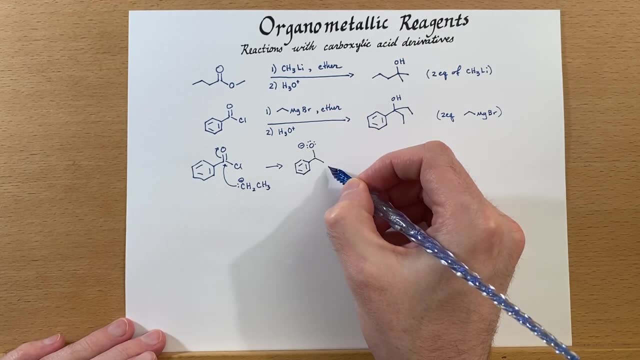 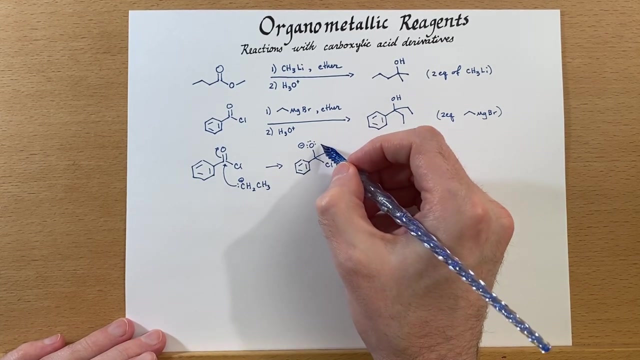 Which will probably be very shortly lived. So negative, charge up on the oxygen. Chloride's here, Grignard reagent now bonded to the carbon there. Now we'll collapse this back down, just like a lot of the other reactions that we've explored. 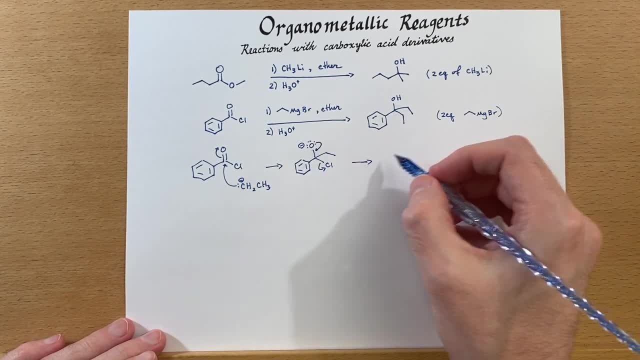 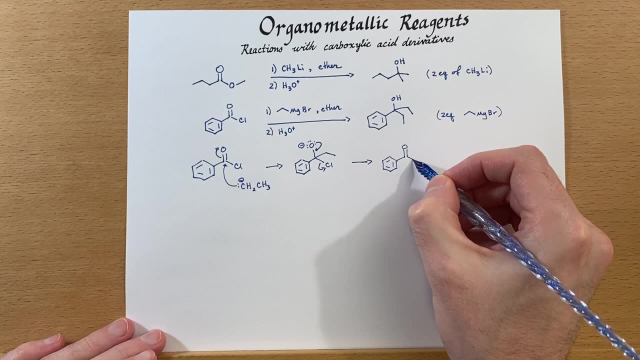 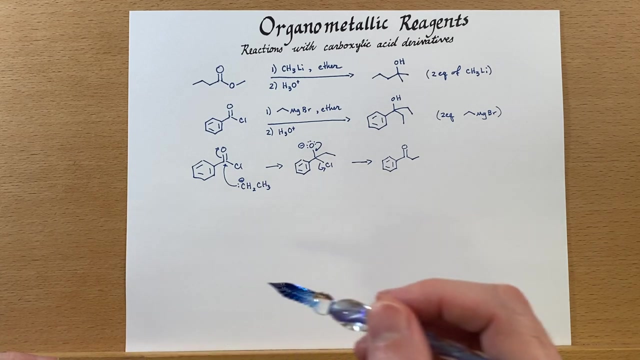 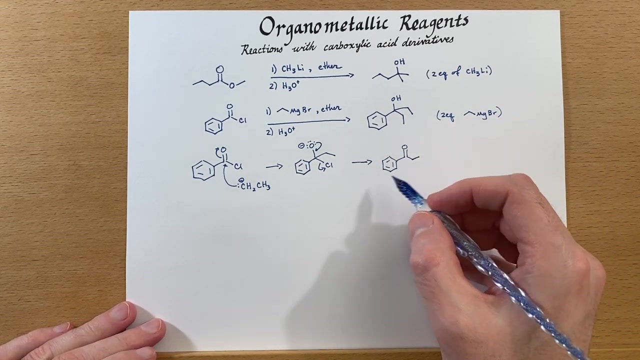 And in this case we will form a ketone Like: so: Now there is additional grignard in the reaction, And so we have a ketone And grignards react with ketones, So we're going to further react this. 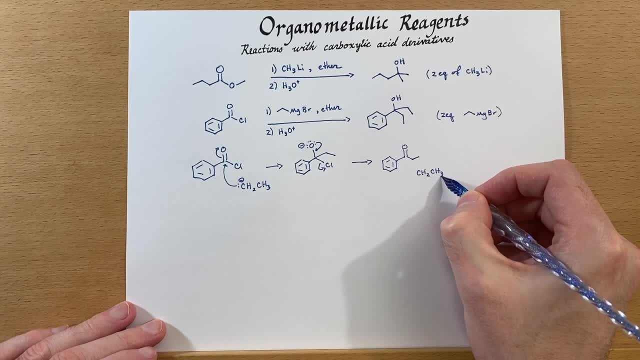 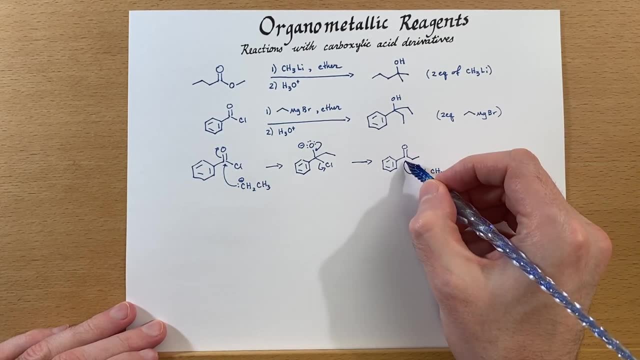 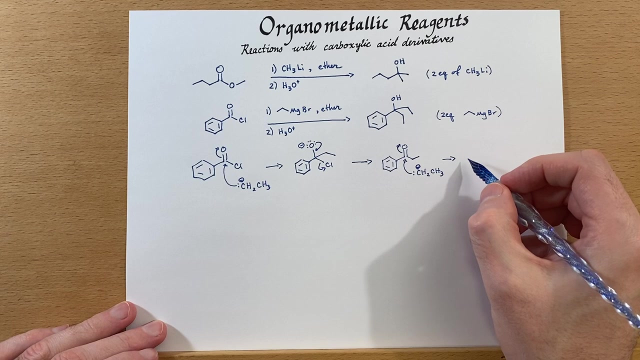 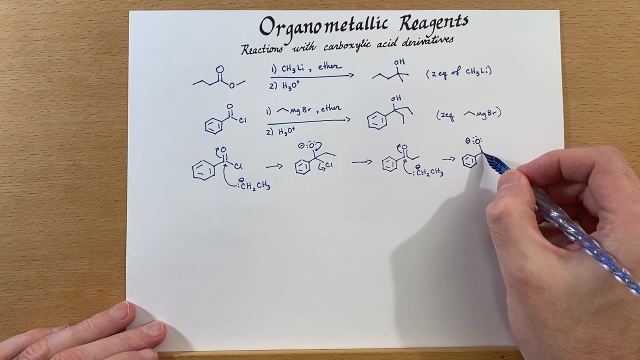 So if we wanted to isolate this material using the Grignard or the alkyl lithium, it's not the best choice because it will attack that carbonyl And again move the electrons up onto the oxygen, And then at this point we don't have any other leaving groups that could depart. 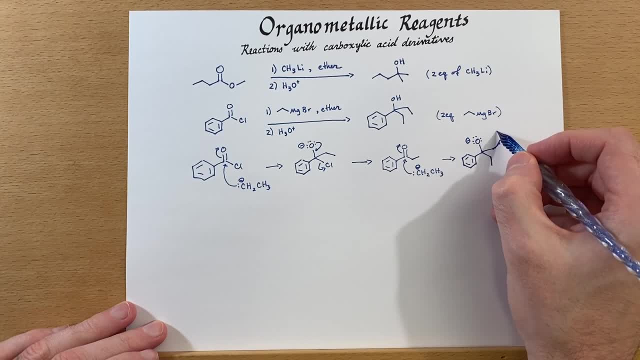 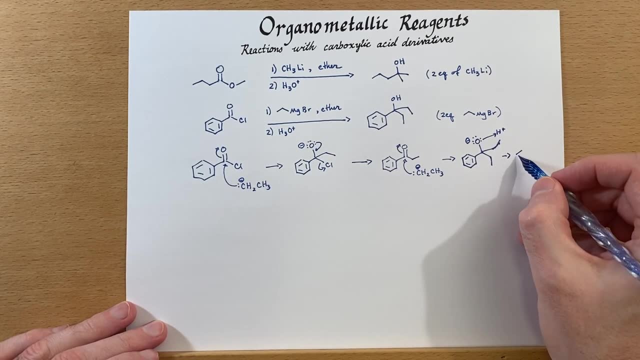 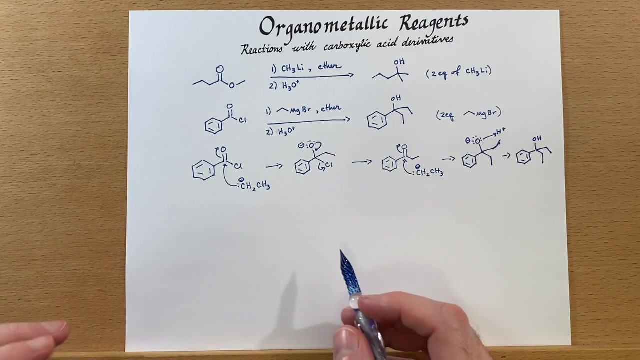 And so we'll just be looking at our acid workup step. So there's our H plus it's going to bond with it And then we form our alcohol product. like so Now: in general, alkyl lithium and Grignard reagents will produce tertiary alcohols from. 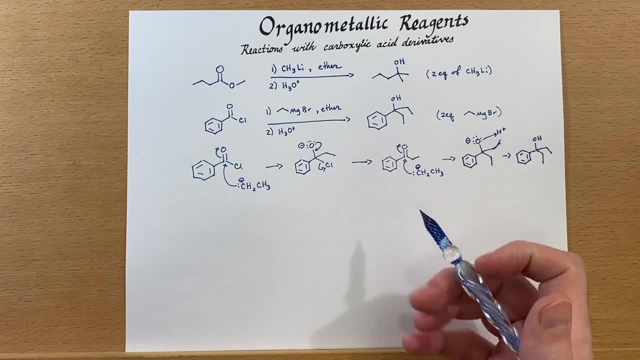 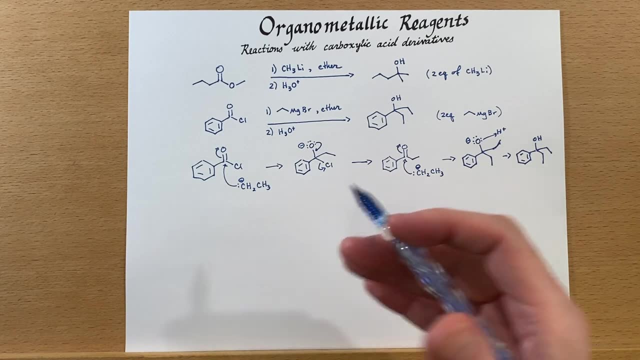 acid chlorides, acid anhydrides, which is an example that I did not show, but it was a certain form. I'll show you in just a few minutes. But this is a birth form of a deal. also react with acid anhydrides and esters. 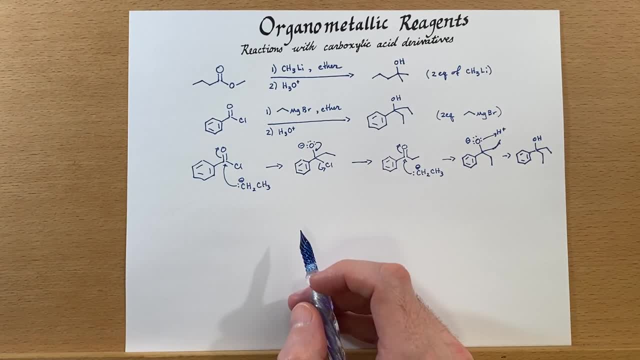 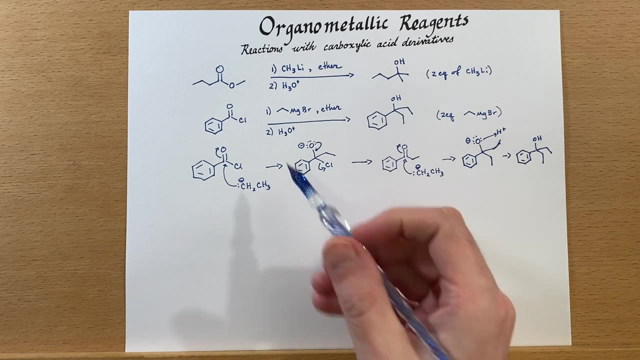 We will not see that reactivity from carboxylic acids because they're acidic and it will destroy the organometallic reagent before other reactions can happen. Also, amides are much less reactive than the these groups: esters, acid, anhydrides and acid. 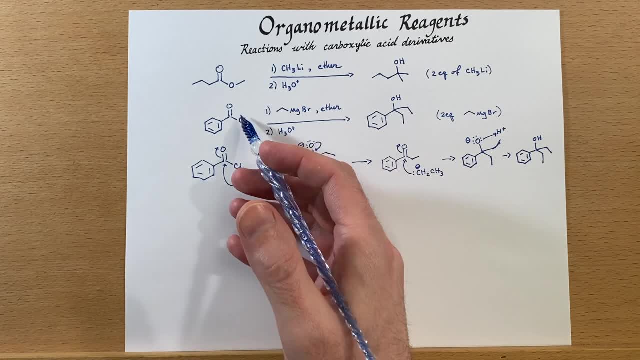 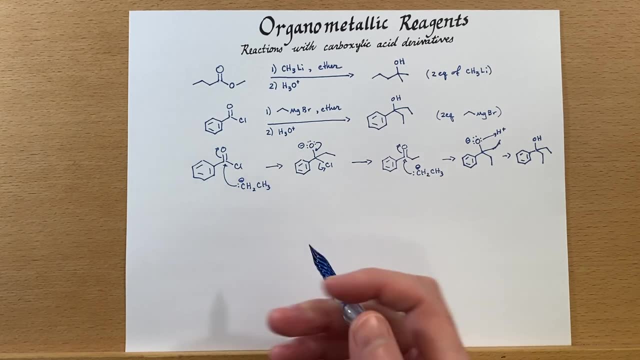 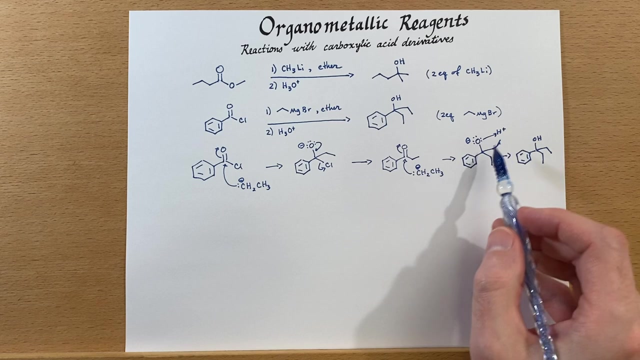 chlorides, So we won't see that reactivity. So three more. Here's our acid. Okay, chlorides, and so they do not react readily. They are also somewhat protic, so you'll have difficulty there as well. Now, I mentioned that this ketone will continue to react and 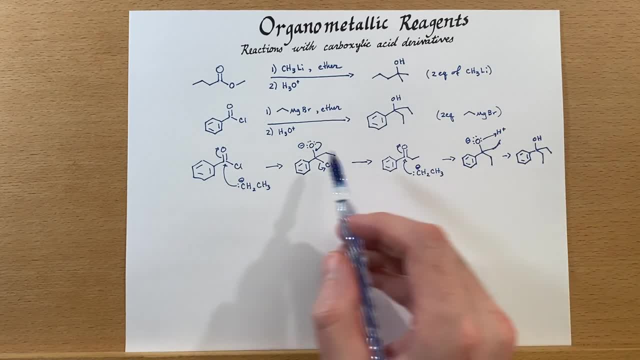 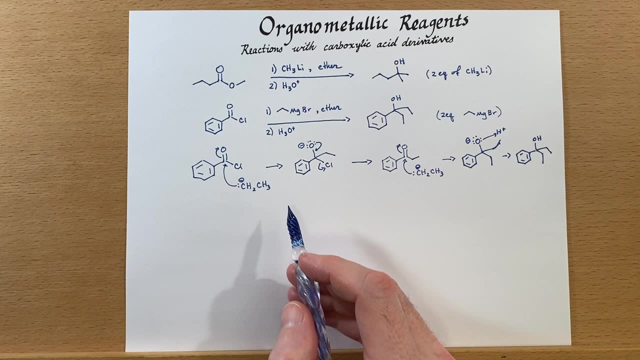 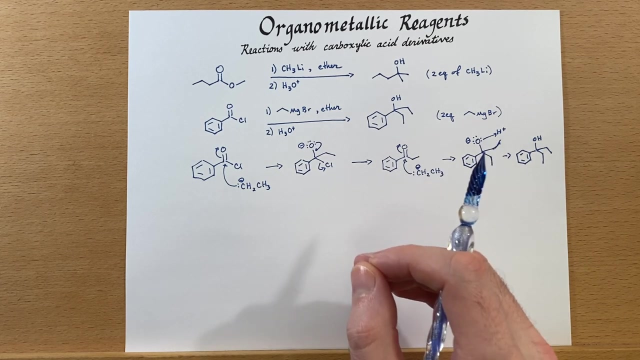 form, the tertiary alcohol, and of course the same mechanism is applying up here with the ester reacting with our alkyl lithium. But what if we wanted to stop at the ketone? Well, there's a reagent that we could use. We need an organometallic reagent that is not as nucleophilic, not as 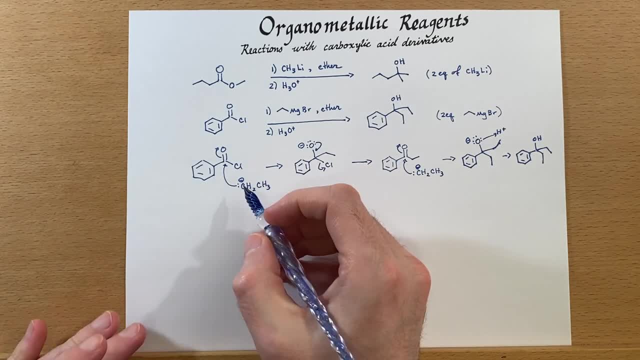 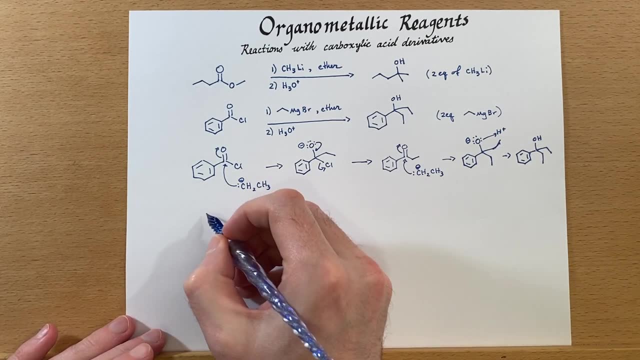 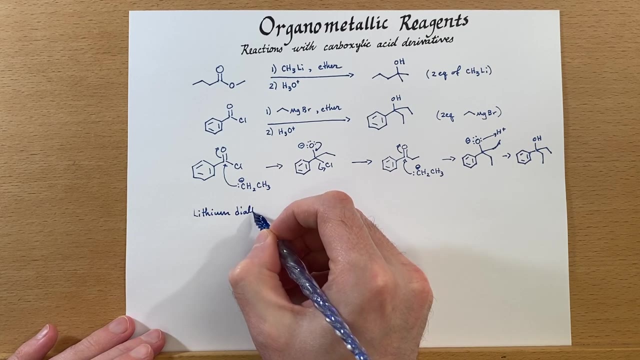 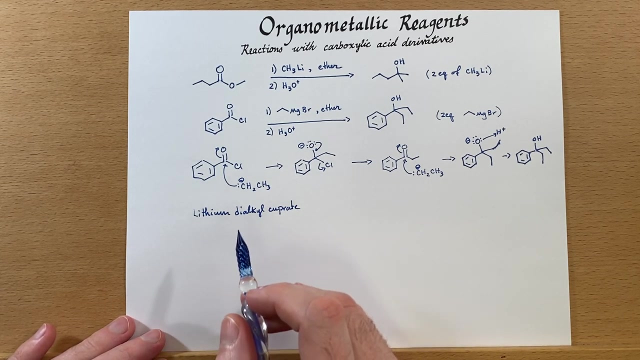 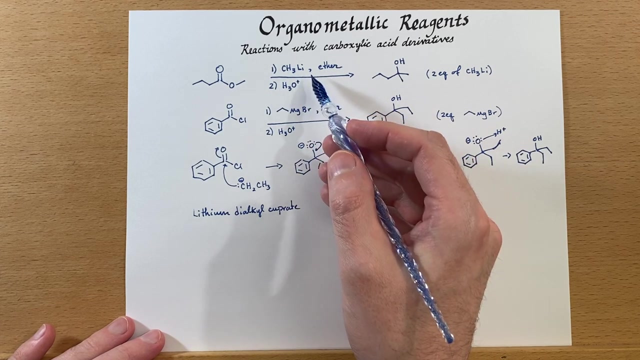 strong and we've talked about one of these before. It's our lithium dialkyl cuprates. So if we were to choose a lithium dialkyl cuprate that will react with acid chlorides- the most reactive out of all of these choices that we've delineated- that will react with these. 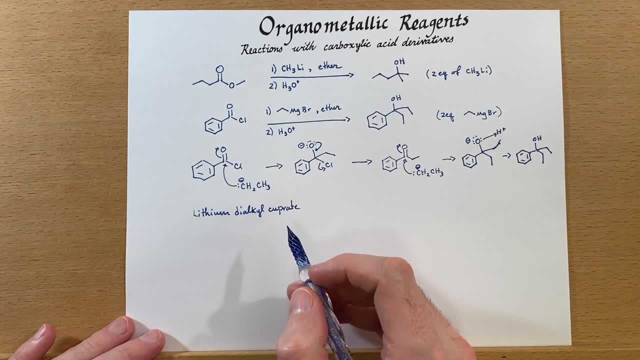 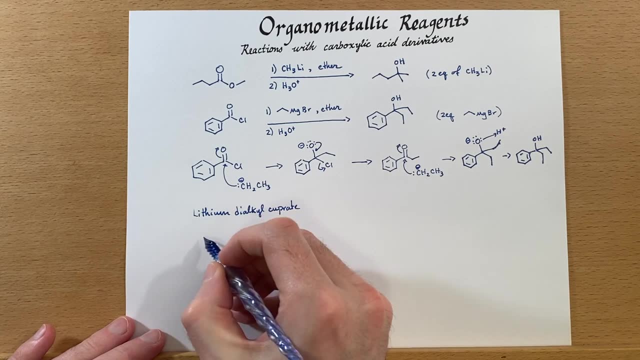 other more powerful Organometallic reagents. It will not react well with esters or acid anhydrides. So if we go back to our benzoyl chloride, which is an acid chloride, and we react this with our 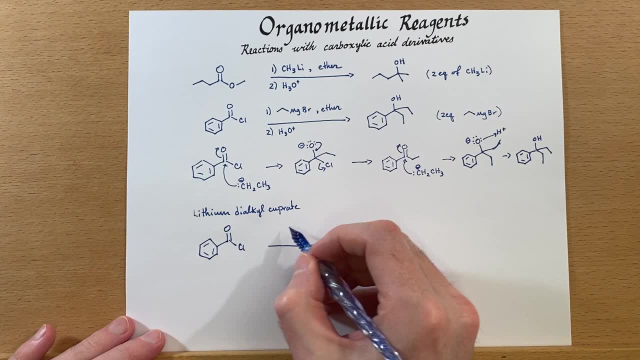 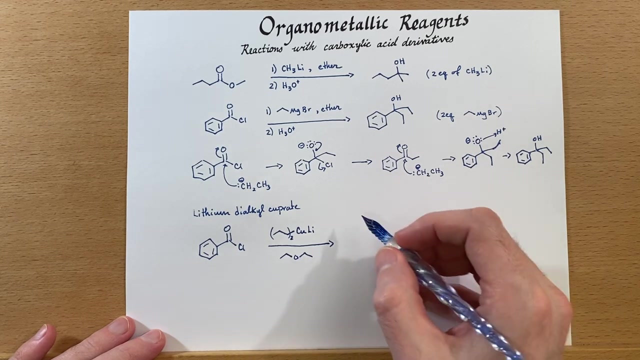 lithium dialkyl cuprate. in this case we'll choose the propyl group. So if we do this reaction, and probably in some ether like diethyl ether, THF, then we'll stop at the ketone Subtitles by the Amaraorg community. 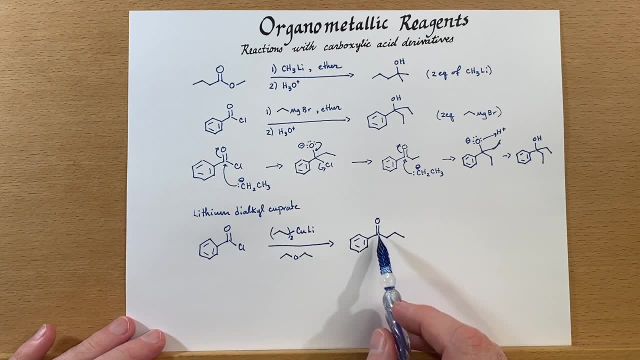 lithium-dioxyl cuprates are just not quite strong enough to directly attack the ketone. Remember these are things that favored 1,4-addition or Michael addition- either way of saying the same thing- and generally left this ketone alone. So we'll see a similar reactivity here, where we have an